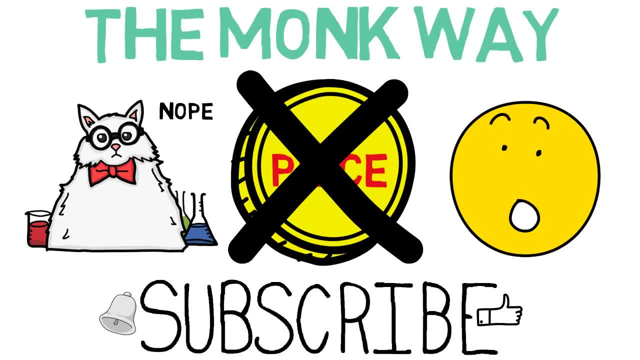 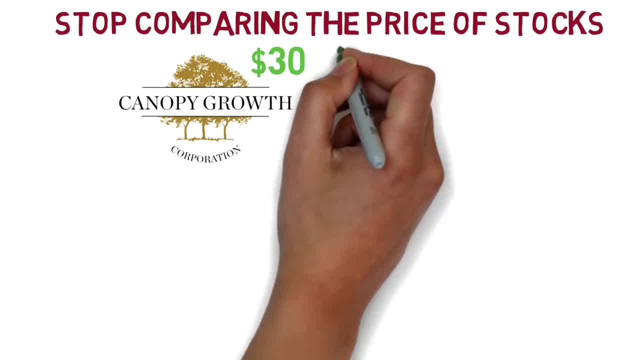 Subscribe and hit that bell for more beginner stock market videos. I make them every day to teach you something new and leave a like if you gain some knowledge. Too often do I find people comparing the price of stocks. recently in my marijuana stocks video- many commenters. 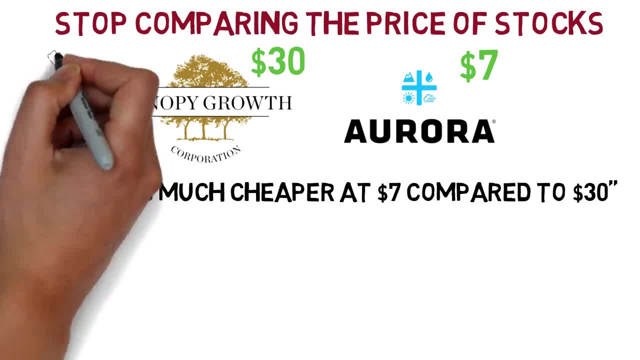 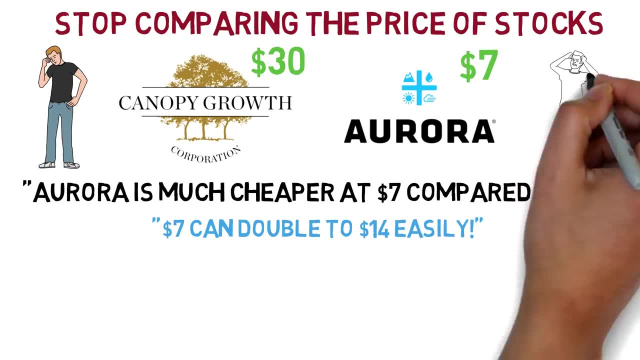 would write something like this: Aurora cannabis is so much cheaper than canopy growth because it's seven dollars compared to thirty dollars, or about how canopy won't double to sixty dollars while Aurora might double to fourteen dollars. this is a very wrong assumption and could lead 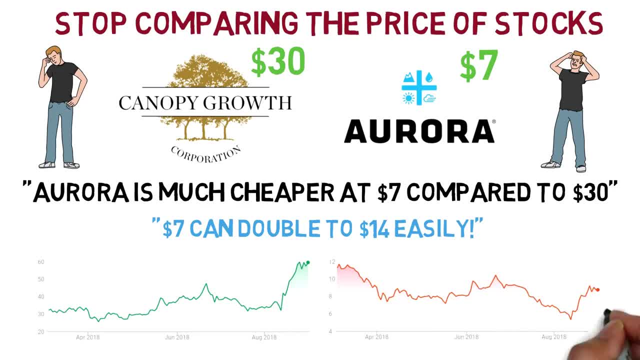 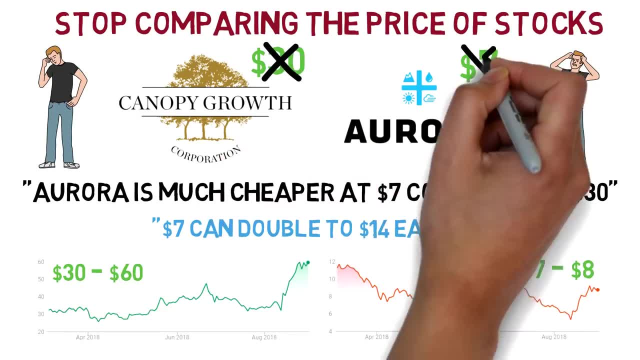 you to buy worse companies. we saw canopy growth doubling in price to sixty dollars, while Aurora went to eight dollars, proving these comments wrong. The price has no bearing at all on how much it can move up or how much value the company has. It's an arbitrary number that can be as high 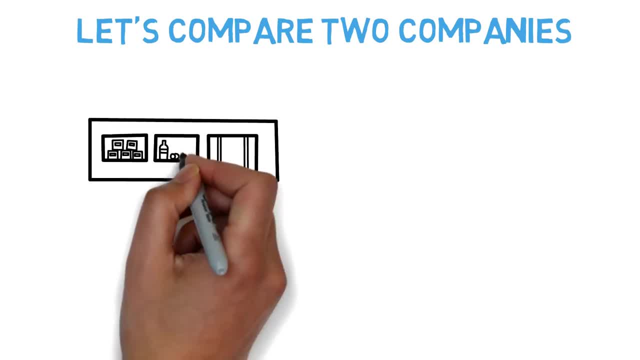 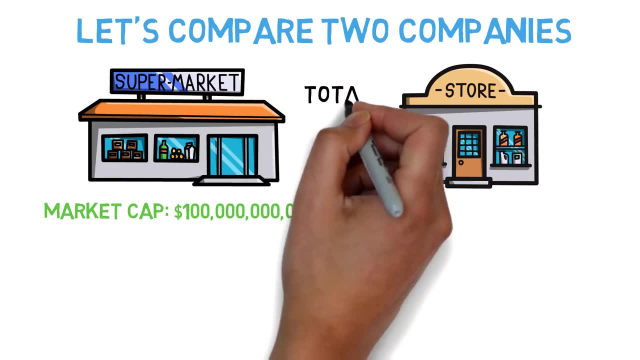 or low as the company wants it to be. To see why the price of a stock doesn't matter, let's compare two companies, company A and company B. Company A has a market capitalization of 100 billion. market cap just means the combined value of all their stocks, so the total value of that company. 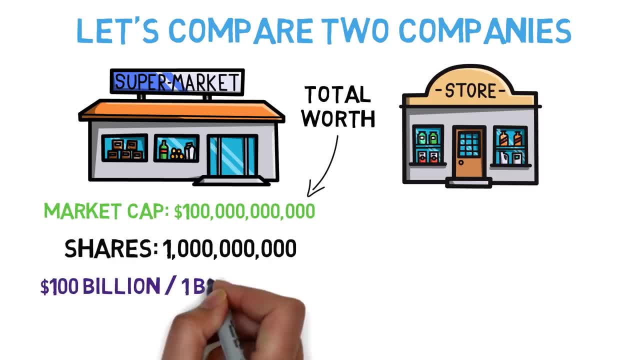 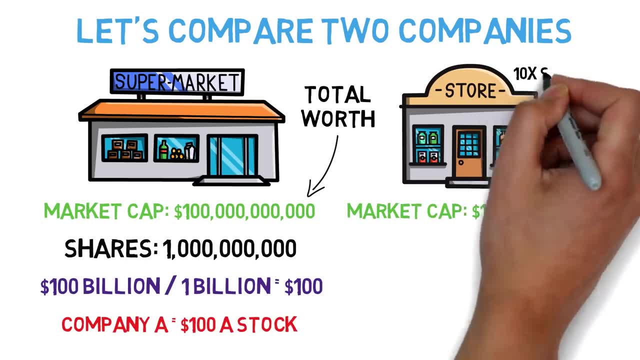 they decided to sell 1 billion shares of stocks during their initial public offering. 100 billion divided by 1 billion is 100 dollars per share. Company B is only worth 10 billion dollars- 10 times smaller than company A, but they decided to sell 100 million shares of stocks. 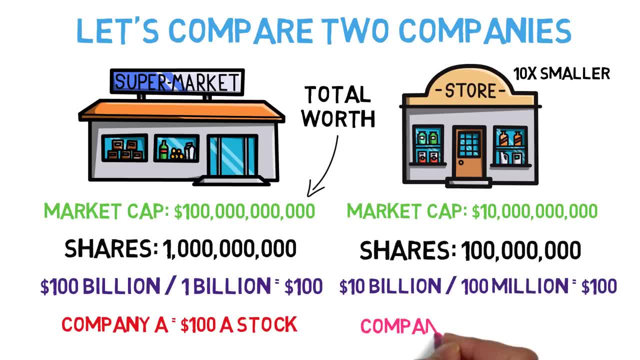 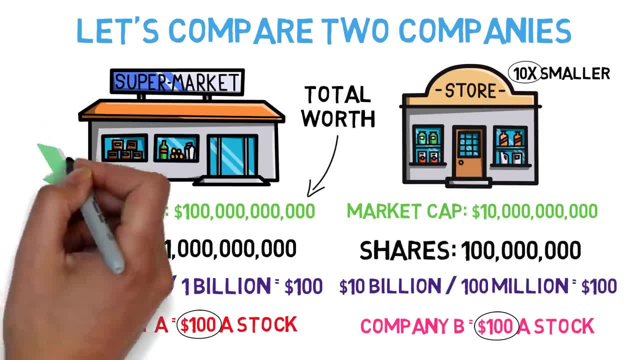 10 billion divided by 100 million is also 100 dollars per share. Does this mean both companies are equal in value, since they're both 100 dollars? No, because company A is worth 10 times as much as company B in market capitalization. Company A is worth 10 times as much as company B in 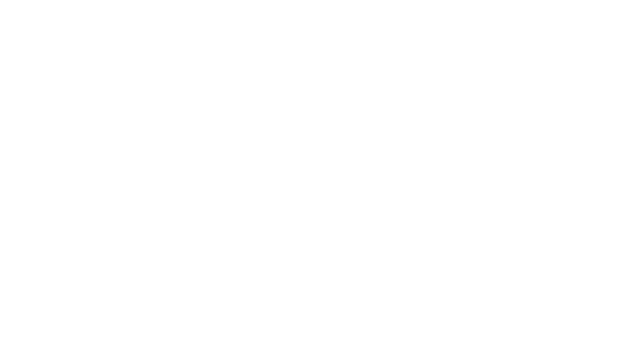 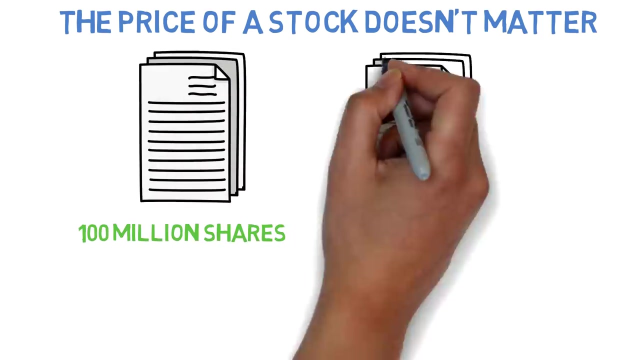 market capitalization. This is why the price of a stock says nothing about their value. The market cap is the important number when comparing company size. The price of a stock is determined by how many shares of stocks the company decide on. Some companies knows that a smaller price has. 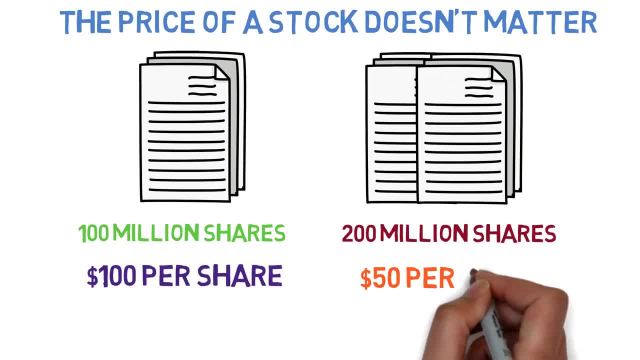 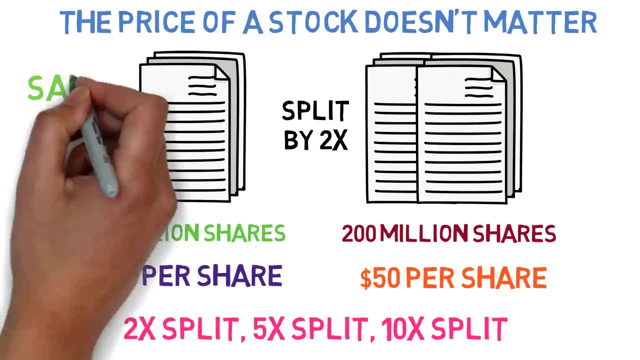 a psychological effect on new investors, They might wish to split the number of stocks they have. If a company decided to split their stocks into more pieces, let's say by two, then their stock price is halved. The value of the stock stays exactly the same, from 100 dollars to. 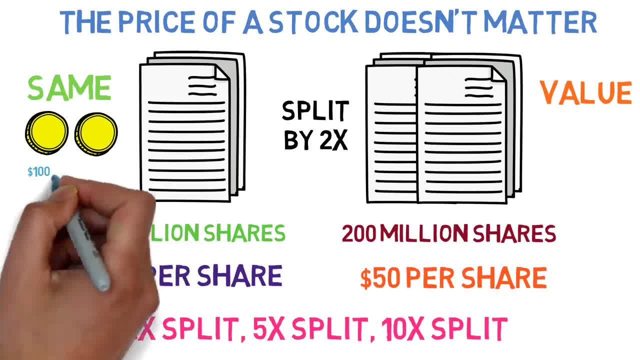 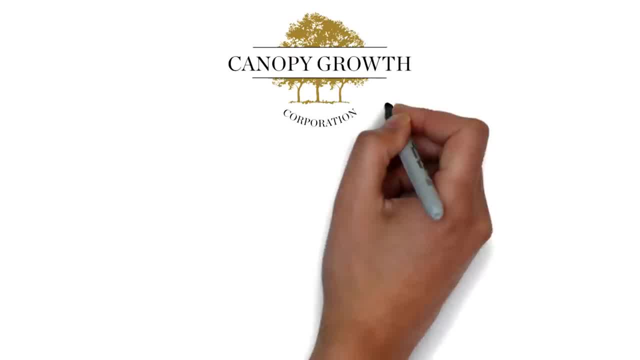 50 dollars, meaning this number is completely meaningless. A 100 dollars stock that makes 100 dollars a year is the same as a 50 dollars stock that makes 50 dollars a year. Canopy Growth was thinking of splitting their stock from 30 dollars to 10 dollars. In this situation, the new investor, 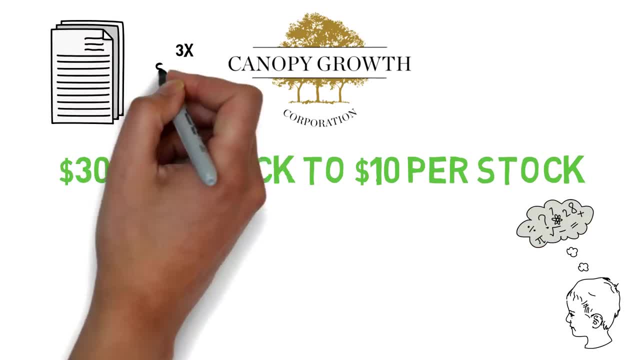 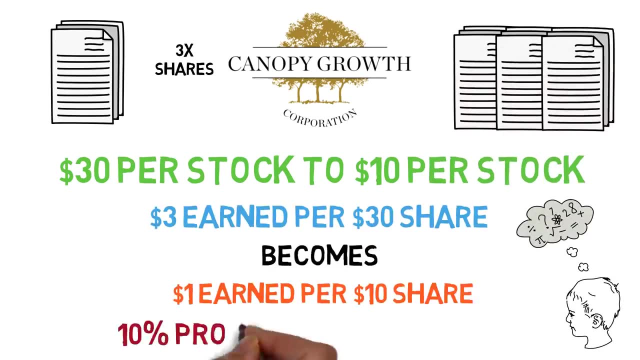 might think they're much cheaper, even though no value has changed. Their price to earnings ratio stays the same because even though the price was cut three times, their earnings per share is also cut three times. This means a company can make their stock price any number they want, If Google. 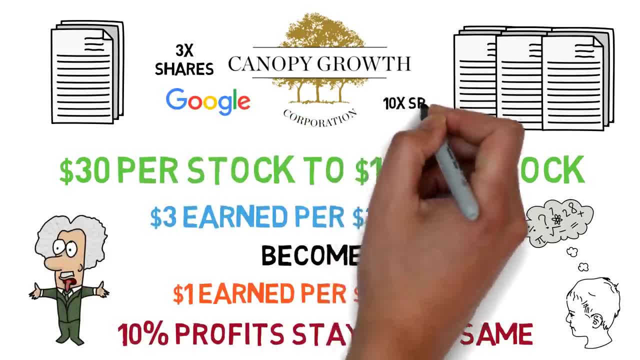 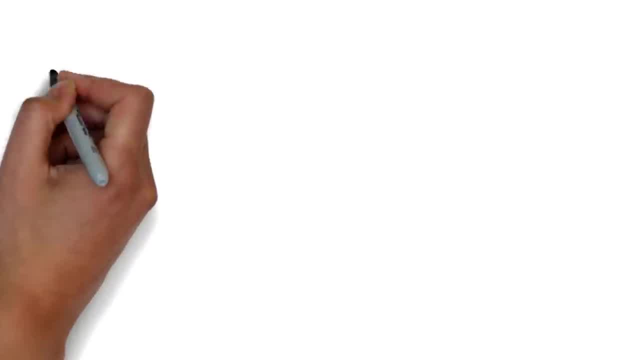 wanted to reduce their price to 100 dollars. they can do this with a 10 times stock split. Companies might do this to get a bigger looking price or a smaller looking price. Nothing has changed except the public perception of their stock. Let's use a real-world example to see why price really. 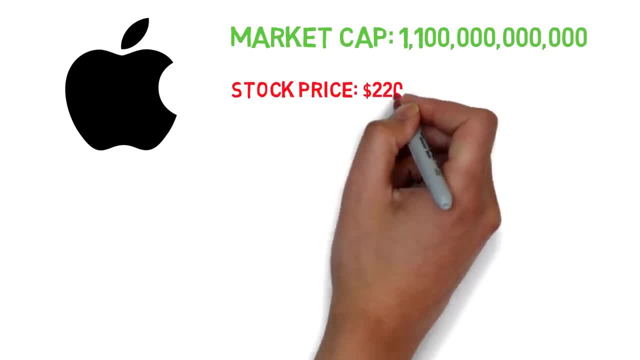 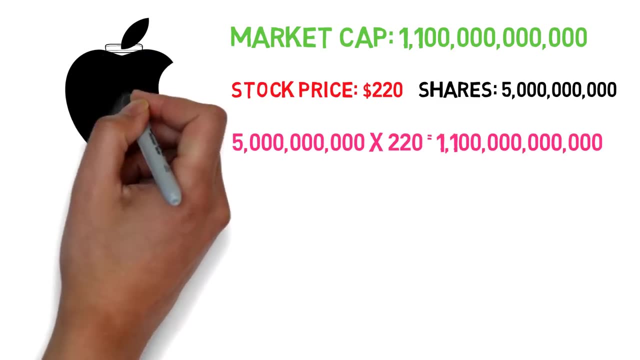 doesn't matter. Apple recently reached 1 trillion dollars in market cap. Their stock price is only 220 dollars, but they have 5 billion shares of stocks. 5 billion times 220 a share is over a trillion dollars, making them the biggest company in the world. A beginner might see this: 220 dollars. 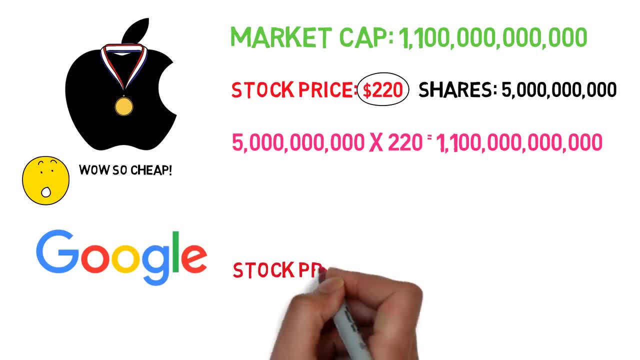 and think this is much cheaper than Google. Google is over 1000 dollars right now, But using what we learned, we can see Google's market cap is 800 billion- 20 percent smaller than Apple, While Apple is only 5 times as expensive as Apple. You can see why the stock price is not important when comparing these companies. Google costs more per stock but is worth less than Apple overall. If these two companies made similar amounts of money, their stock price should go up at the same rate, Meaning Google might go up 20 percent in a year from 1000 dollars to 1200 dollars And Apple might. 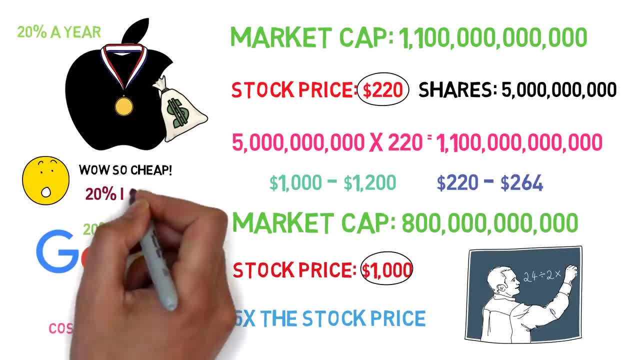 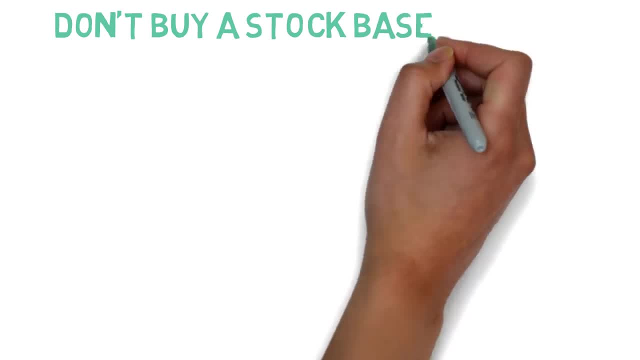 go up 20 percent too, from 220 dollars to 264 dollars. Even though they have a big difference per stock, they would go up at the same rate if they had the same amount of value and profits. Don't buy a stock just because it has a lower price than another similar company. 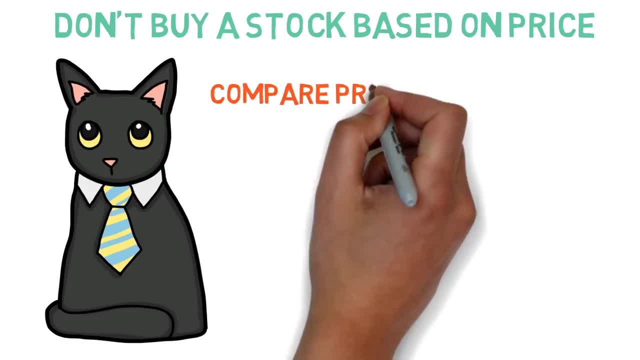 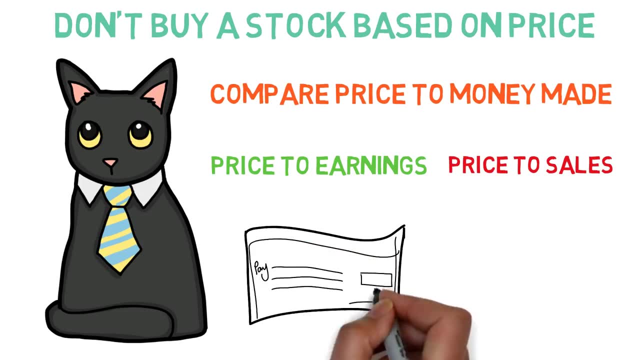 The real way to determine value is comparing their price to how much the company made in cash and profits. This is why we have the price to earnings ratio and the price to sales ratio, Because the price is not an important number, but comparing it to how much they made. 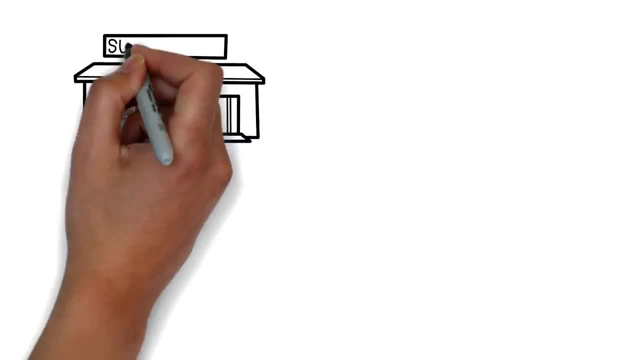 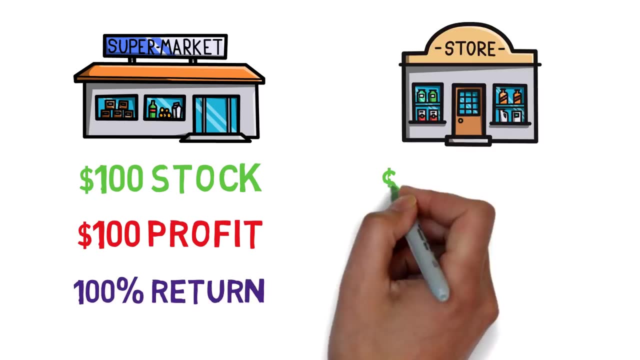 gives us the real value of a company. For example, if company A is 100 dollars a share and they made 100 dollars per share in a year, this is a return of 100 percent a year. And if company B is 10 dollars, but they only made 1 dollar per share a year, 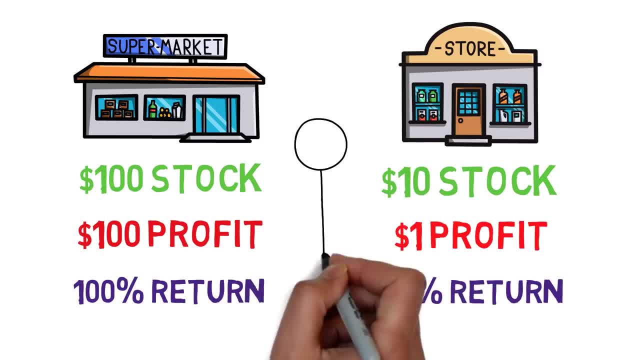 this is a return of 10 percent a year. If you had 100 dollars, which company would you choose? The beginner might buy 10 shares of company B, thinking it's a cheaper stock and having more shares feel better. This would be a mistake, because the market can see their earnings. 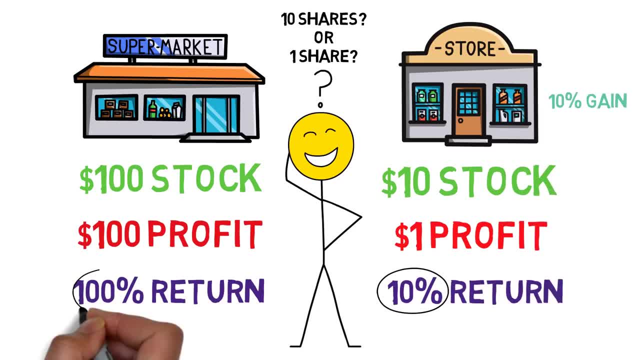 of 10 percent a year and might only raise the stock price by 10 percent in that year, While company A, even though they cost 10 times more per stock, is making much more money and might give you 100 percent in that year. The beginner might have made 10 percent on. 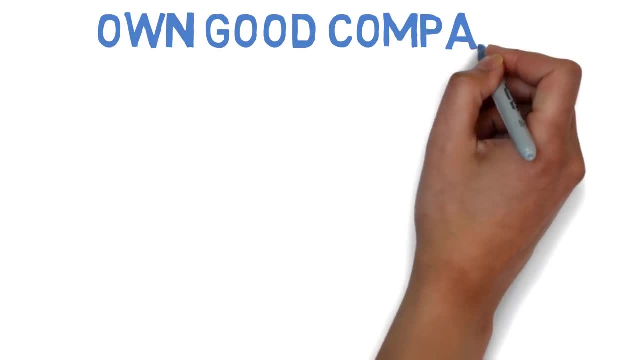 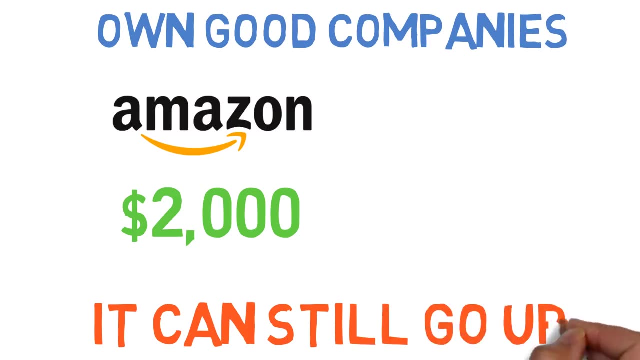 his investment, missing out on 100 percent in returns. with company A. This means it's better to own 1 share of a good company than 1000 shares of a lower value company. Amazon just reached 2000 dollars. this might seem expensive. 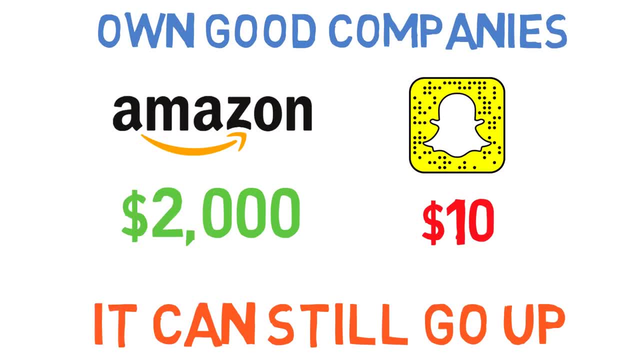 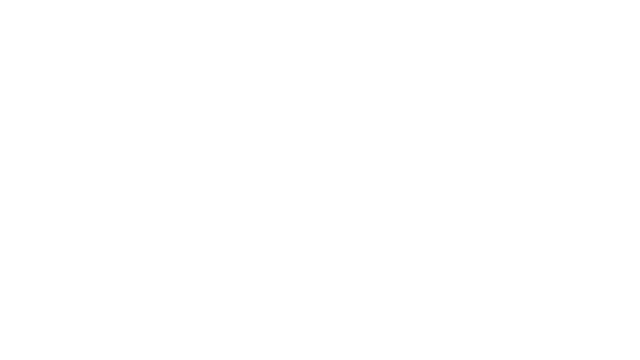 but it doesn't mean it can't keep going up. It's much better to buy 1 share of this than 200 shares of Snapchat at 10 dollars. Amazon actually makes money and increases users, while Snapchat loses money every year and has problems keeping users. 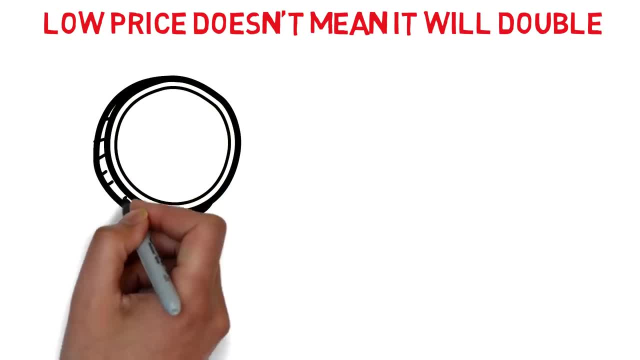 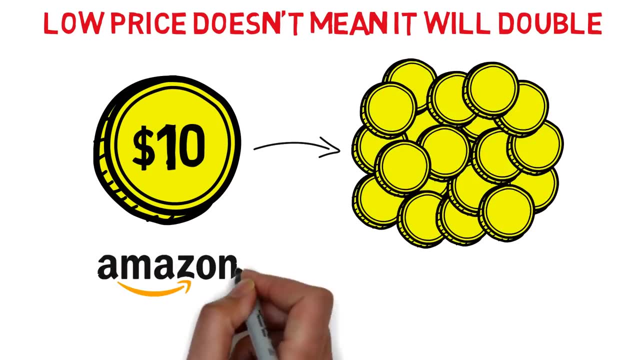 People tend to think lower priced companies has more room to go up. A common thought is a 10 dollars company is much more likely to double to 20 dollars than a 1000 dollars company doubling to 2000 dollars. This is not true either. we saw Amazon going from 1000 to 2000 in less than a year. 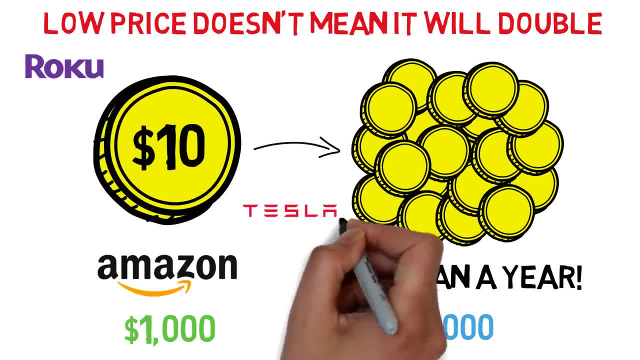 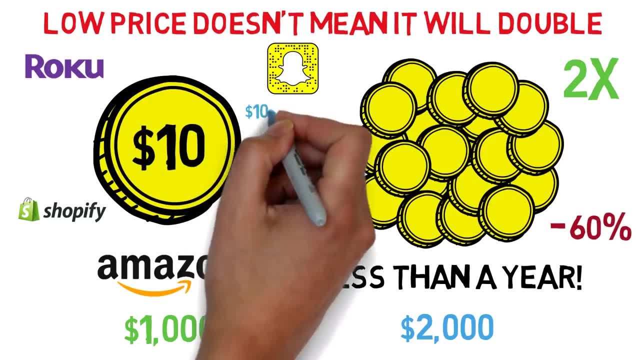 but this might happen more to lower priced companies because they tend to be high volatile risky stocks, Meaning there's more chance of them doubling, but also more chance of them dropping 50 percent or more. For example, we saw Snapchat move from 10 dollars to 14 dollars, then back to 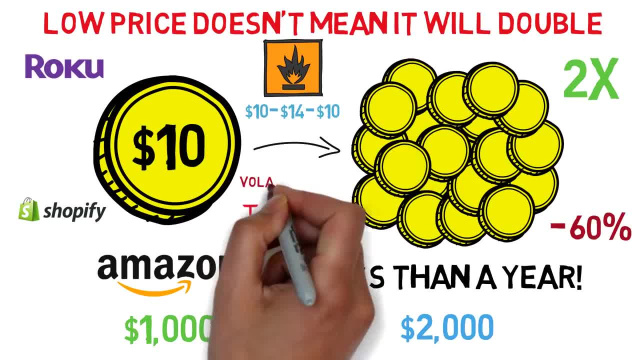 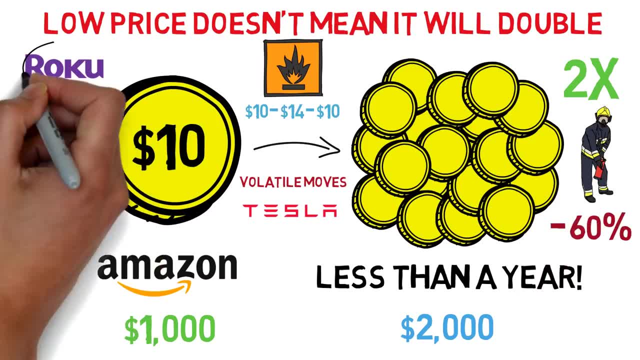 10 dollars in a short time. This isn't because their stock price is low. this is because it's a volatile company without profits. lower market cap companies tend to have lower stock prices. these companies are more risky in general. A small company worth a few million has more of. 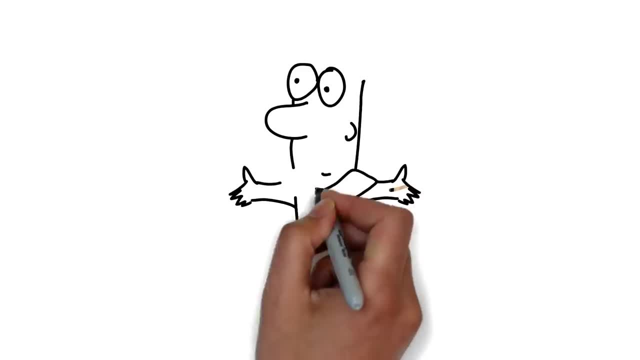 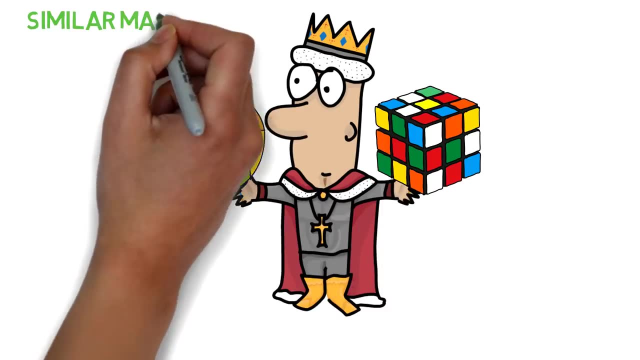 a chance to double than an old and established company like Google. The next time you see 2 similar companies and 1 is 3 times as expensive, Don't assume that means it's costing you more- more money If they're making the same amount of money with similar market caps. 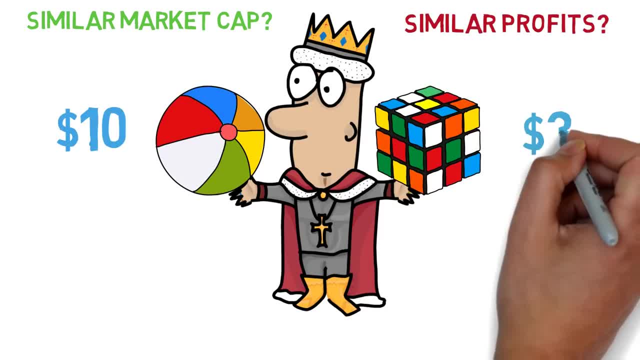 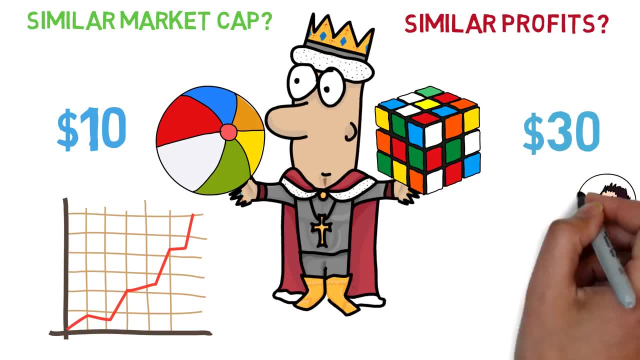 it means they will have similar worth. So a 10 dollars company might be worth the exact same as a 30 dollars company. they can both go up at the exact same rate. The only time stock price should matter is if you can't even afford to buy 1 share of that company, for example, if you're. 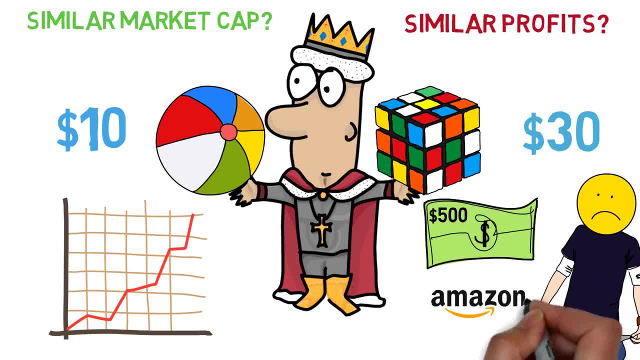 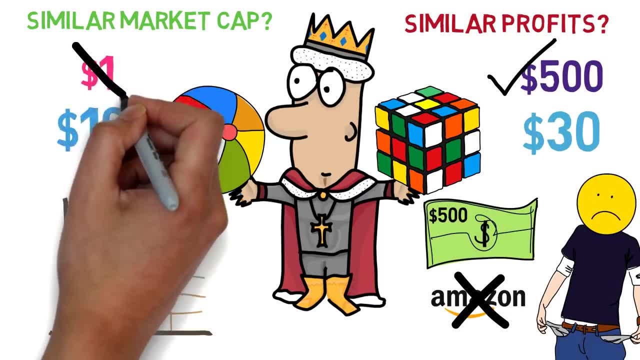 really new and you only have 500 dollars, then you can't buy Amazon. In that situation you should still understand. buying 1 share of a 500 dollars company might be better than 500 shares of a stock. that's a dollar. Owning a million shares of a dying company doesn't mean anything but owning 1. 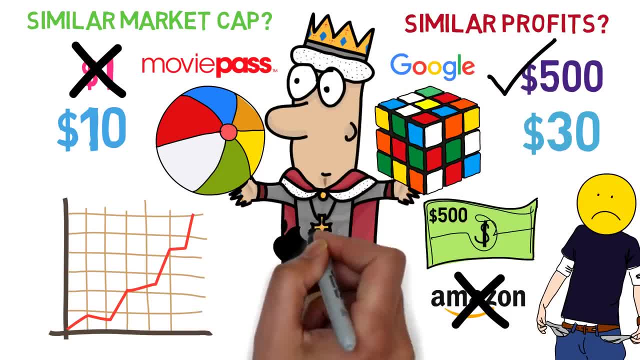 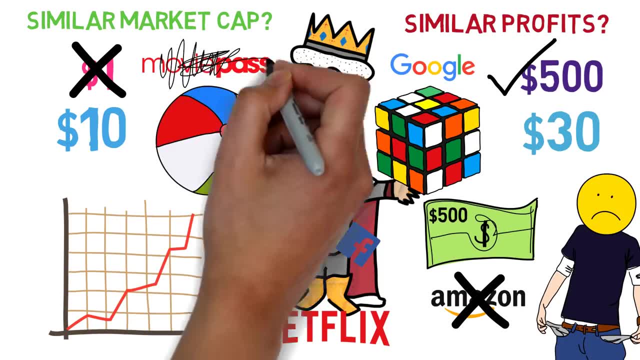 share of a big company like Apple or Amazon means you get a slice of a great company. You must remember when you buy a stock you own a piece of that company. so don't buy a stock of a company you wouldn't want to own. do your research to find the real value of that stock. 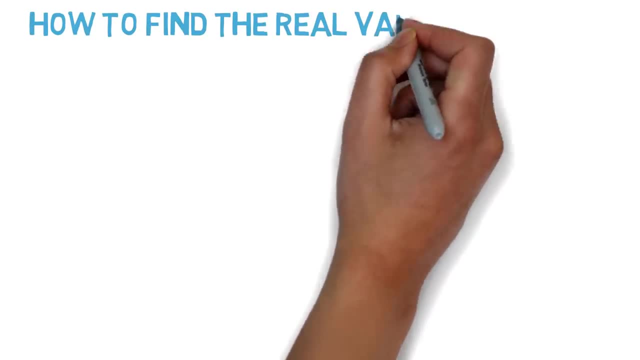 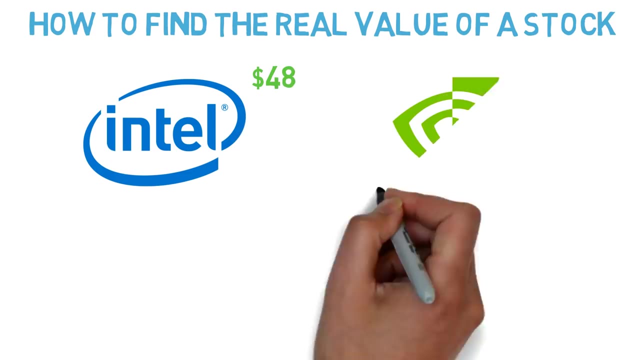 before any purchase. Let's look at another real example to really understand this and to see how to actually find the value of a company. Intel is a blue chip company. everyone knows They're trading at 48 dollars. Nvidia is also a chip maker known by gamers for their graphics cards. 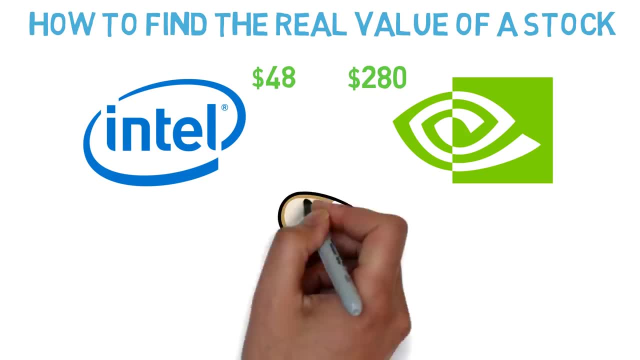 trading at 280 dollars. Using what we've learned, we can see that so far, we don't know which company is a better value or which is more expensive, Even though Nvidia looks like it's 6 times more expensive. this is not how stocks work. Looking closer at their market cap. 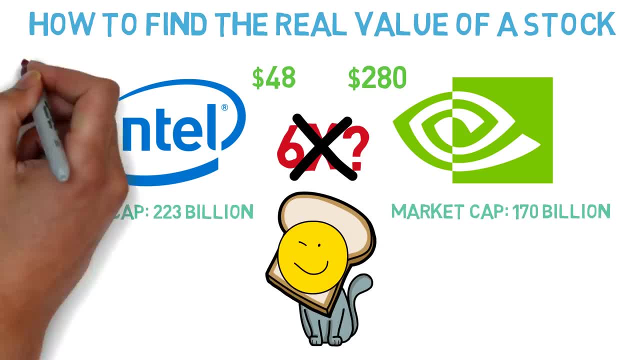 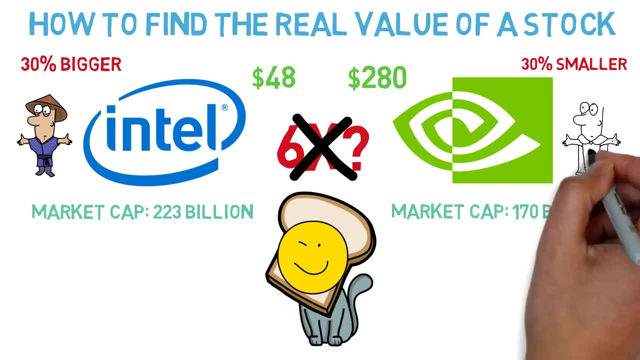 the combined worth of all their stocks together, we see Intel is 223 billion, while Nvidia is 170 billion. This means Intel is a bigger company, even though they're 5 times cheaper per share of stock. but this still doesn't determine their worth. When buying a stock, we have to compare that. 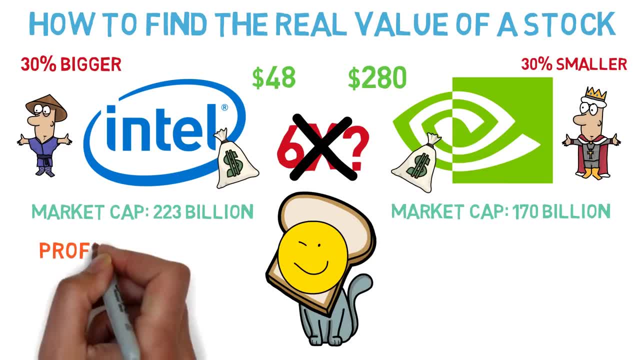 market cap to how much they made per year. For example, if Intel made 223 billion last year, while having a market cap of 223 billion, they made 123 billion. If the market sees this, they might increase the stock by 100% because of this crazy growth. 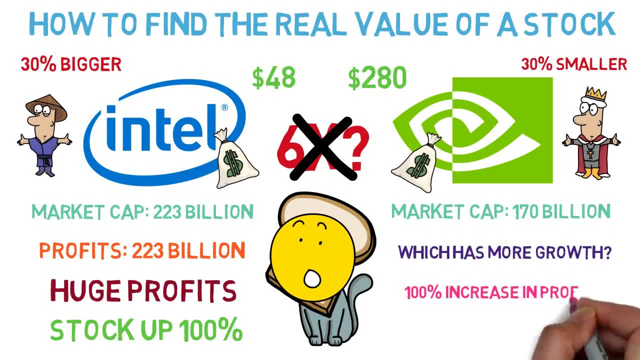 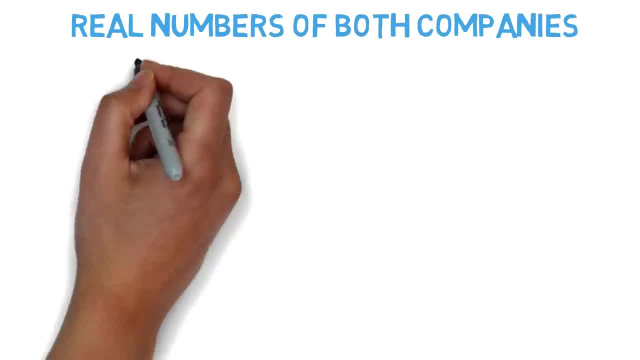 When we look for a stock, we have to look for the one with more growth. A huge spike is usually because a stock made more money than last year and 100% increase in profits might move a stock up 100% once the numbers are released. In reality, Intel has a P? E ratio of 17.. 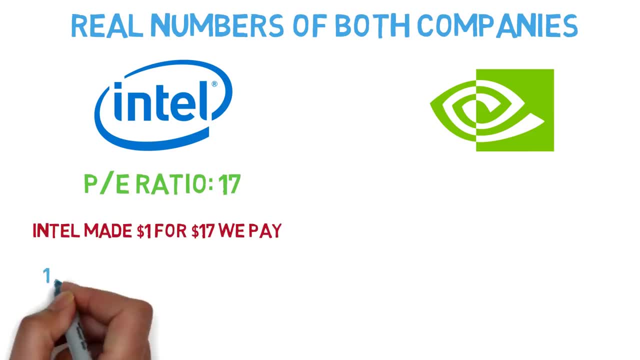 This tells us they made 1 dollar for every 17 dollars we're paying. Dividing 1 by 17, we get the percent they made in the past year: 5.9%. This means we can expect them to make 5.9%. 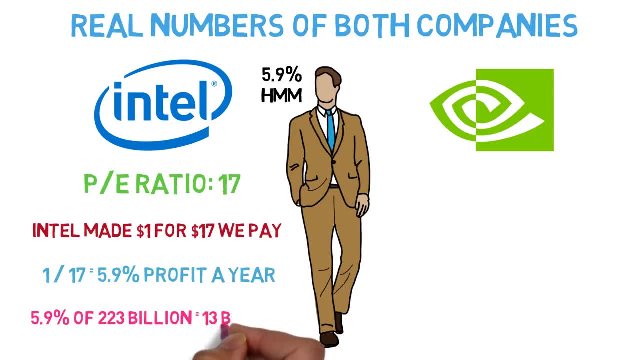 of their worth back per year, while increasing slowly every year. 5.9% of their 223 billion market cap is 13 billion, so they made 13 billion of profits in the past 12 months. Looking at Nvidia, they have a P E ratio of 41,. 1 divided by 41 is a. 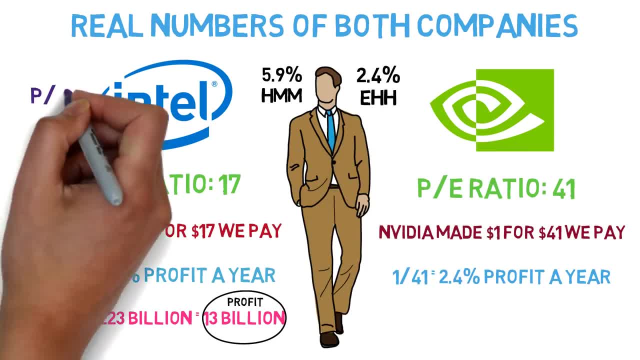 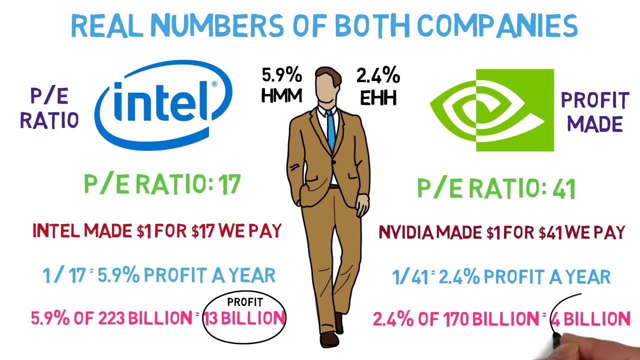 return of only 2.4% a year. This is twice as low as Intel. The price to earnings ratio tells us their profits in relation to their market cap. So 2.4% of Nvidia's market cap of 170 billion is 4 billion, meaning Nvidia made 4 billion dollars of profit in the past 12 months. 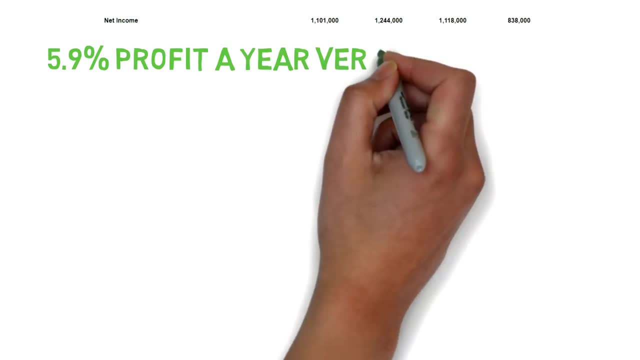 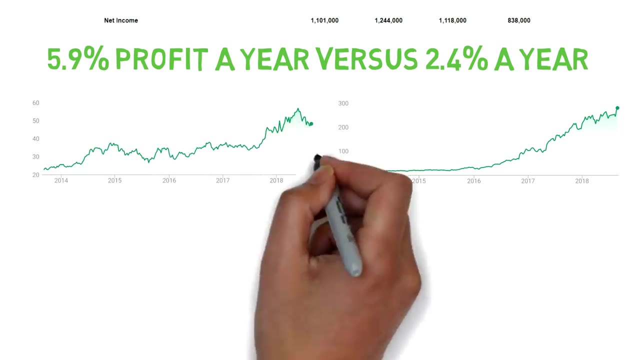 Looking at their income statement, this checks out perfectly. This tells us their real worth. Intel is a better deal because they're making 5.9% a year, while Nvidia is making 2.4% a year. But this is not the whole picture. Intel only went up 100% in the past 5 years, while Nvidia 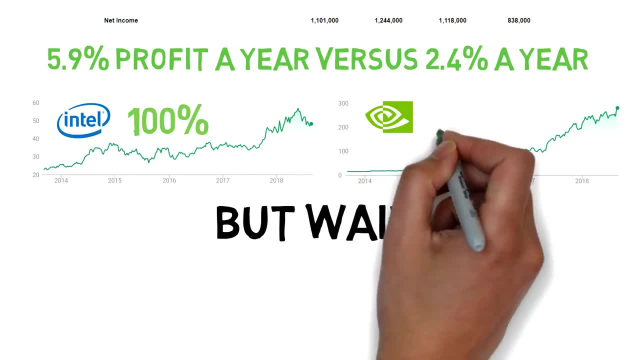 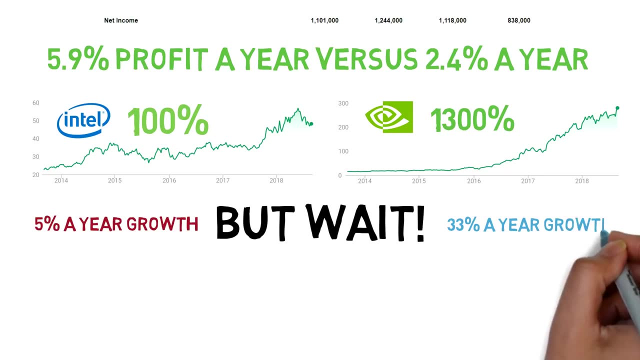 went up 1,300% in 5 years. This is because Nvidia has been growing much faster. Looking at their revenue growth for 5 years, Intel went up an average of 5% a year. Nvidia went up an average of 33% a year. This means a smaller market cap company might have more chances of extremely high.